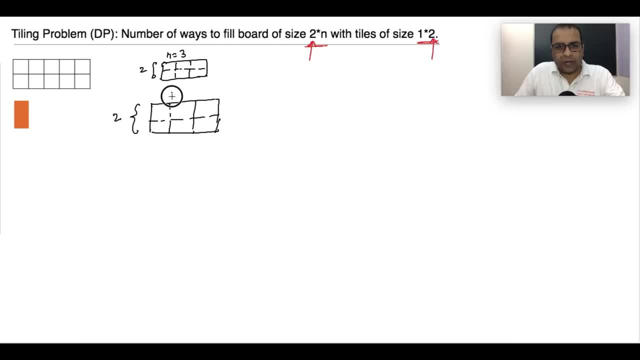 So this is the board. Width of the board is 2 and length of the board is n is equal to 3.. So we place the bricks in a vertical manner. Though the bolts are placed right placement, the set set of the top three level to face 1 and length of the board is 1.. If we place bricks vertically, 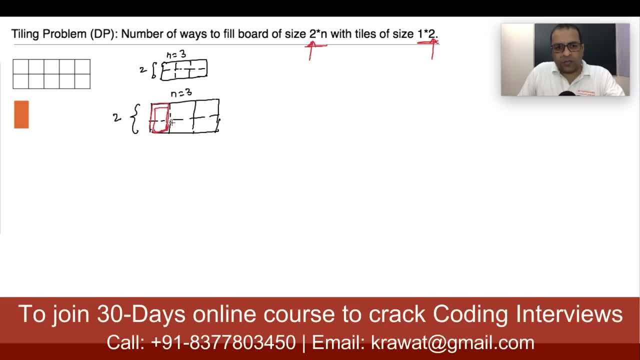 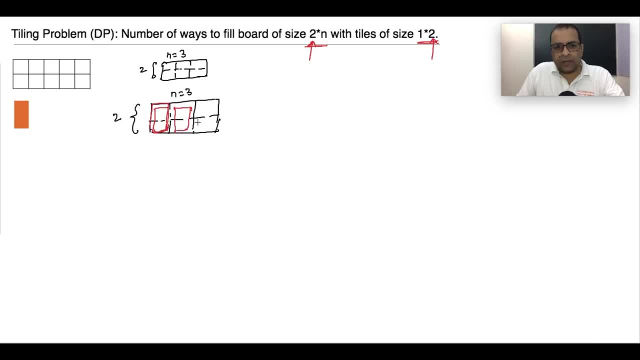 then what we are designing now is drown it out. So one way of like this to place the bricks is and that we can place all the bricks vertically. The bricks will exactly overlap the the first two blocks. I am drawing little smaller bricks So that it is clear that the bricks we are placing the bricks vertically, So the second brick is placed like this and the third brick is placed like this. So this is one of the ways of putting the brick. I am also placing rods next to each other, because this is the quote which is important here. So we want to place more美國石 and the bricks will overlap. Now let us place bricks vertically, So the bonded bricks will exactly overlap the first 2 blocks. So this project Êd. 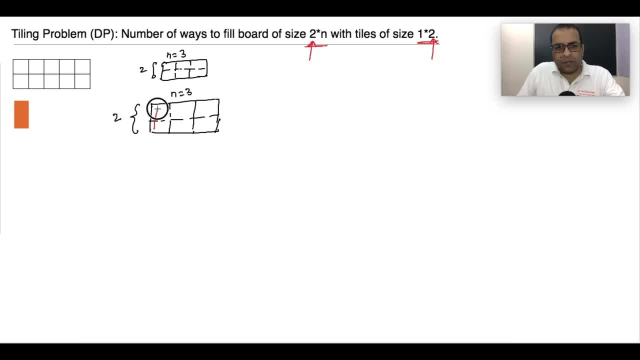 another way can be that I can put the first brick vertically and rest of the two bricks horizontally. yet another way is to put the first two bricks horizontally and then the third brick vertically. similarly, there can be multiple solutions. we want to find total number of ways in which this entire 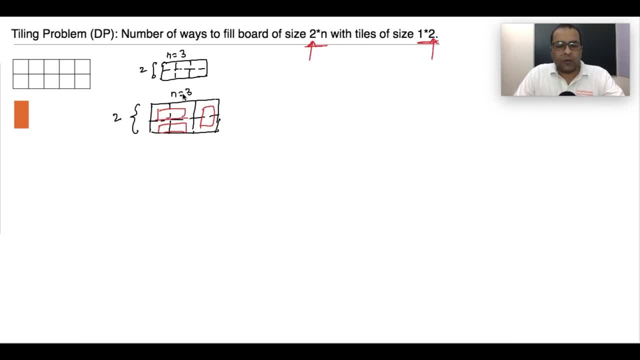 plot or this entire board can be filled. now one thing is clear: that to fill a board of size n- cross 2 with bricks of size 1- cross 2, we require exactly n bricks. no matter how we place the bricks. but we require exactly n bricks because area of the plot is 2n and area of the brick is 2, so total number: 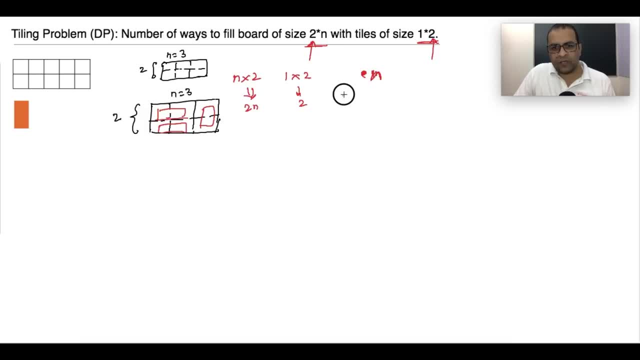 of bricks required to fill the fill. the entire area is obviously 2n divided by n divided by 2, which is equal to 2n to n, right? so there will, there will always be the number of bricks, will all number of bricks required to fill the entire board or fill the entire plot, will always remain constant. we are 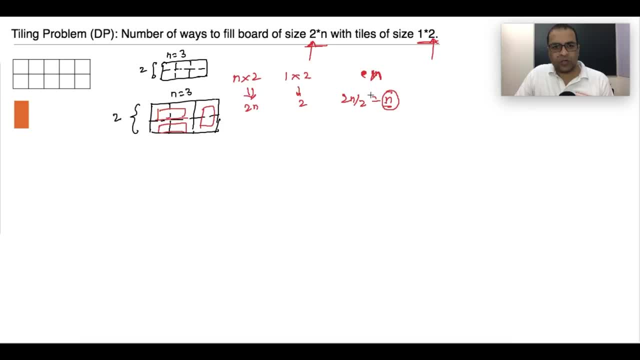 not talking about number of bits, a number of bricks. we are only talking about the arrangement of bricks and we want to find number of unique ways, number of unique arrangements of filling the entire board with bricks. all right, now let us look at the solution. as we have seen, 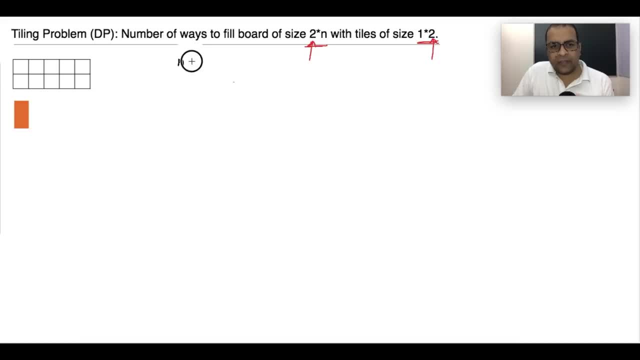 the only variable here is n. n is the length of the board. the width of the board is 2 and dimension of the brick is fixed, which is 1 cross 2, so the function will be something like this. the signature of the function will be integer. number of ways: integer. 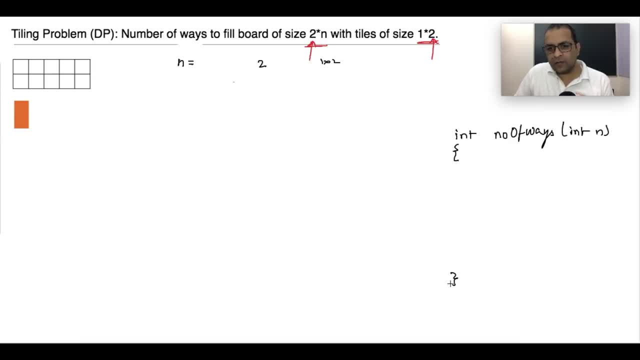 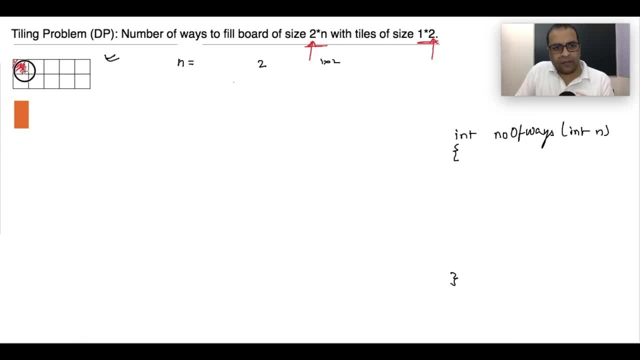 brick vertically, then that brick will occupy this block and this block. now we are left with a board of size n minus 1, cross 2. the width of the board remains 2. the length of the board is now n minus 1. so if we place the first brick vertically, then we are left with n minus 1. 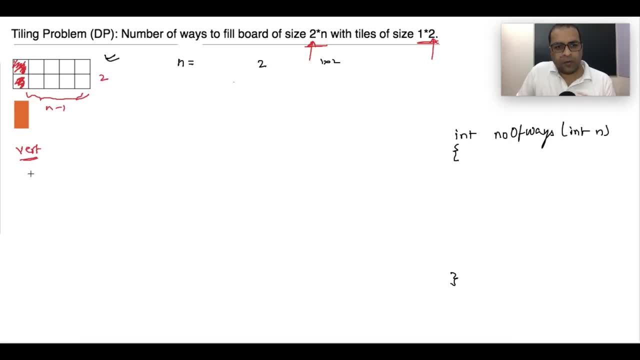 we are left with a board of size n minus 1. so the problem now reduced to find number of ways to fill a board. fill board of size n-1. alternately, we can put the first brick horizontally. if we put the first brick horizontally then the first brick will fill these two blocks. 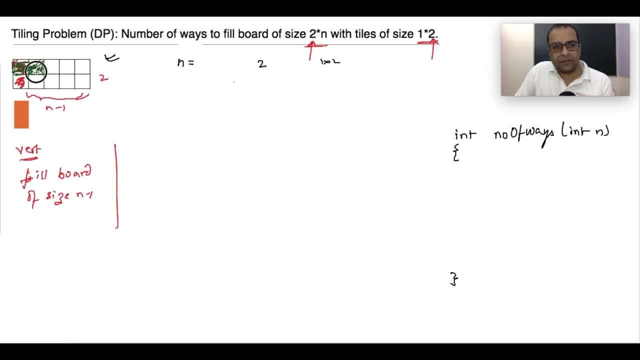 so the first brick will be placed like this and it will fill this area. now, if the first brick is placed horizontally, then the first brick has filled two units in the first row. in the second row, a brick cannot be placed vertically. in the second row, a brick can only be placed horizontally. 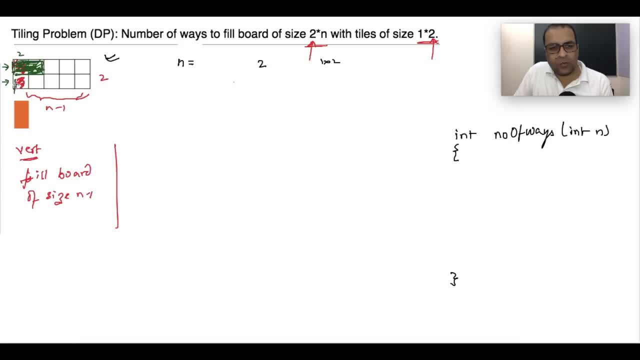 so the way of putting, there is only one way of putting the second brick, which is horizontally in the second row. so if we place the- let me just repeat it- if we place the first brick horizontally in the first row, then there is only one way of putting the second brick. 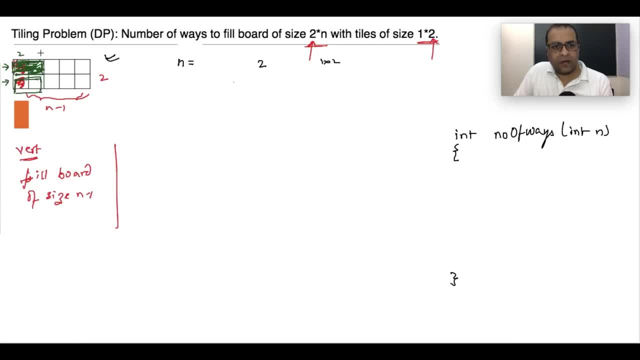 brick in the second row, which is horizontally. after putting these two bricks, we are left with a board of length n-2 to be filled. so if we have placed the first brick horizontally, then it forced me to place the second brick horizontally below it, which covers the board of size n-2. 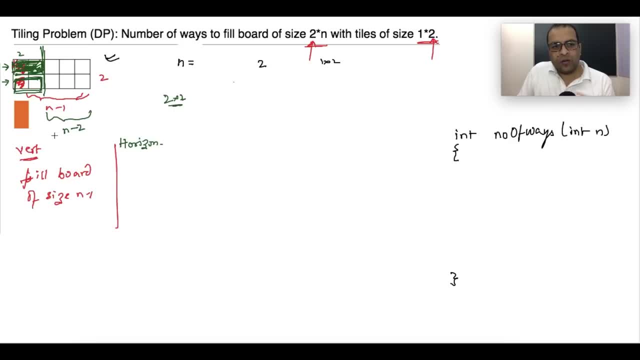 which covers the board of size 2x2, and now my problem is reduced to find number of ways to fill the board of size n-2. so in a board of size n i can either place the first brick vertically or i can place the first brick horizontally. 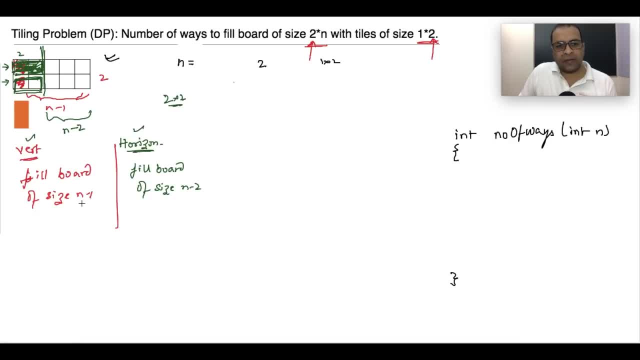 there is no other way. if i place the first brick vertically, then i am left with a board of length n-2. if i place the first brick horizontally, then i am left with a board of size n-2. so total number of ways. total number of ways. 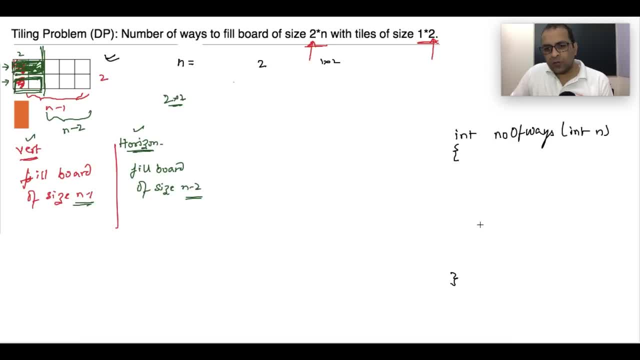 to fill a board of size n is equal to total number of ways. number of ways of filling a board of size n-1 plus number of ways of filling a board of size n-2. so this will be the value and we will just return this value. 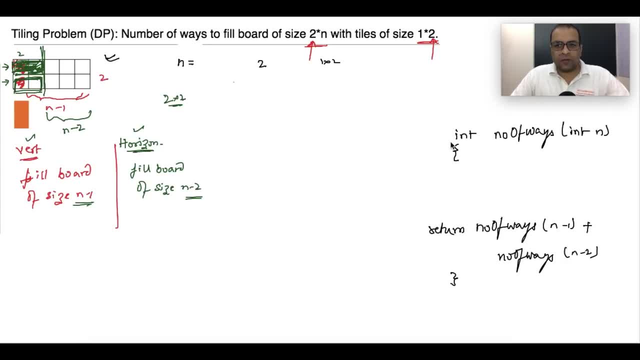 so we have defined the recursion, and that is the beauty of recursion. we know that recursion comes with lot of drawbacks. recursive function takes more time. recursive function takes more memory. but recursion is such a powerful tool, especially in the interviews. recursion can be used to solve really complex problems. 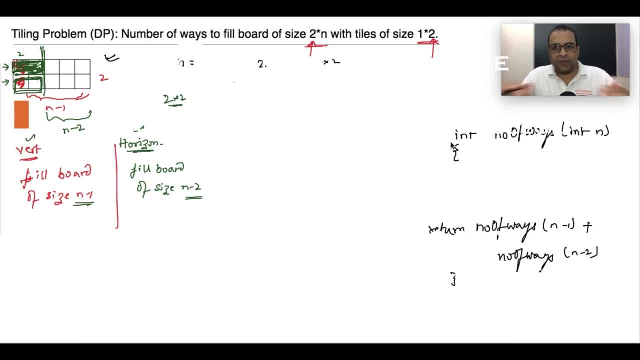 in a really easy way. so the challenge here is that we are given a larger problem. we just need to define the larger problem in terms of smaller problems. maybe we are given this larger problem as we are doing it here, so we are just moving on here. so we are just moving on here. 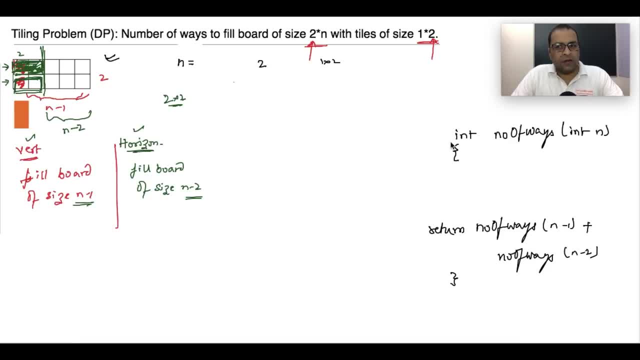 so we are just moving one step forward. by moving one step forward, we are left with a sub-problem which is of the same type, and those sub-problems can be solved recursively. now let us put a terminating condition, otherwise the recursion will be infinite recursion. what will be the terminating condition? 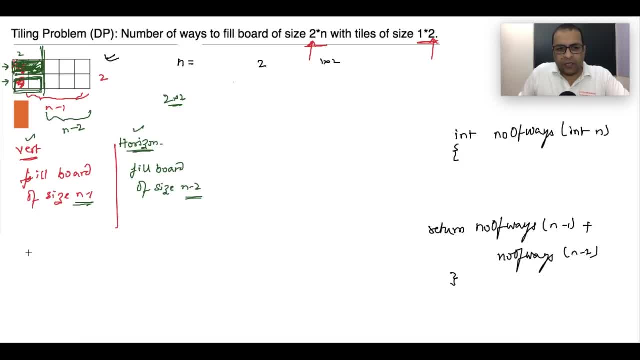 to find the terminating condition we need to find. the solution for n is equal to 1 and n is equal to 2 because we are moving up to the depth of n-2. solution for n is equal to 1 means that the size of the board is 2 cross 1. 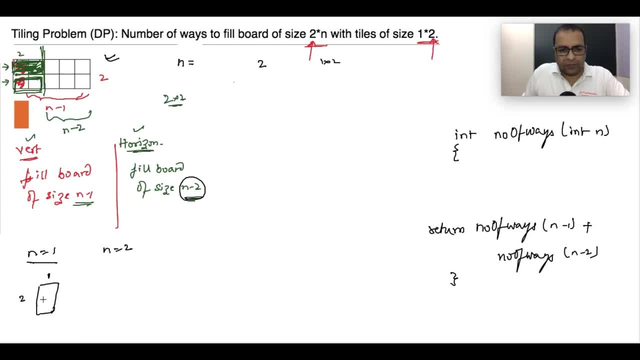 the width of the board is 2 and the length is 1, so n is equal to 1. there is only one way of putting a tile in a board of size 2 cross 1. when the size of the brick is also 1 cross 2. 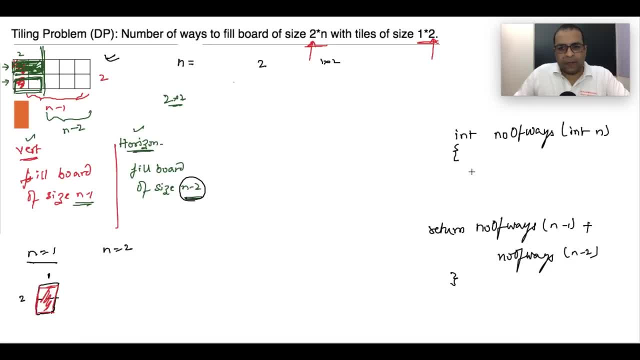 so the brick can only be placed vertically. there is no other way. so that will be our first terminating condition. if n is equal to 1, then return 1. now what if n is equal to 1?? if n is equal to 2, means the width and length of the board are also 2. 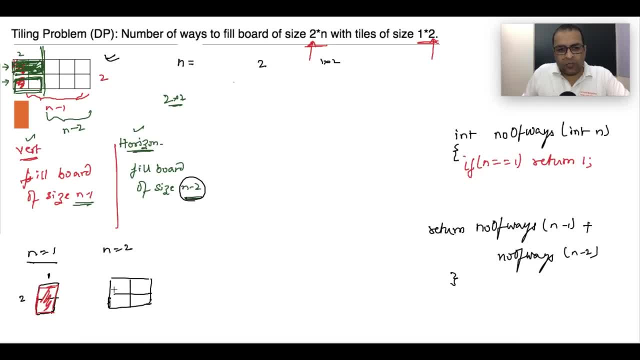 so if the length and length of the board is also 2 and width of the board is also 2, then there are two ways of putting a brick of size 2 cross 1. one way is that we can place both the bricks vertically. another way is that. 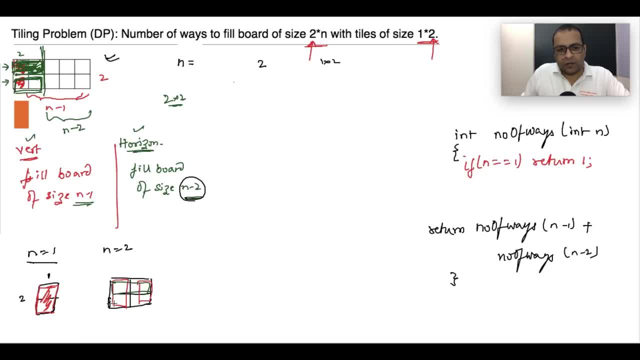 we can put both the bricks horizontally. so if we put the first brick horizontally, then we have to put the second brick horizontally, and if we put the first brick vertically, then we have to put second brick vertically. So there are two possible ways. So if n is equal to 2, then return 2.. 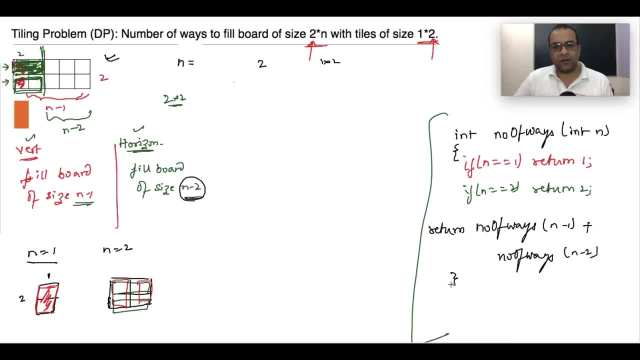 Now, if you look at this solution carefully, then this solution is that to solve a problem of size n, the solution of a problem of size n is equal to sum of n minus 1th term and sum of n minus 2th term. 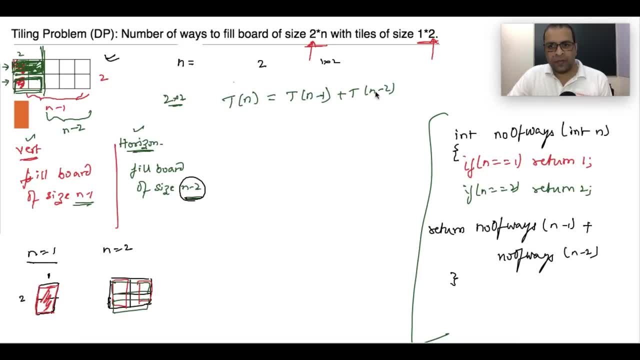 I am saying term in a loose way, Basically to kind of relate this problem with Fibonacci series. Now the solution is exactly same as Fibonacci series. nth term of Fibonacci series is equal to sum of n minus 1th term and n minus 2th term. 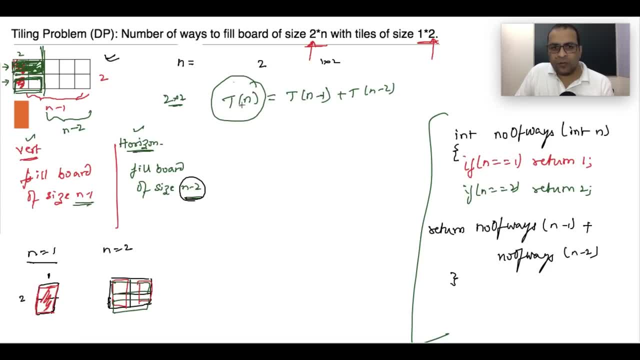 Here also, solution of the function with n is equal to 6 is equal to. solution of the function with n is equal to 5 plus 5.. So it is exactly same, except maybe for the terminating conditions. In Fibonacci series. the first two terms are 1 and 1.. 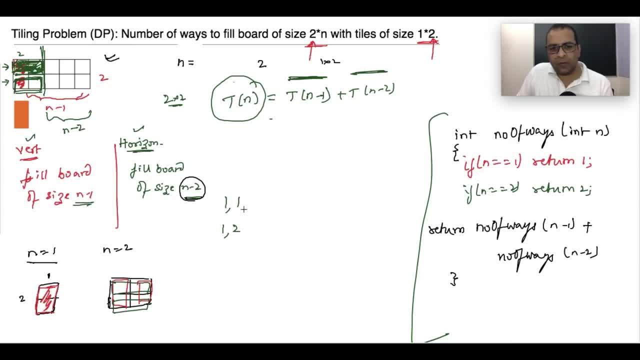 Here the first two terms are 1 and 2.. So if the length of the board is 3,, then third term of Fibonacci is 2.. Here, if the length of the board is 3, then number of ways of putting the bricks will be 3.. 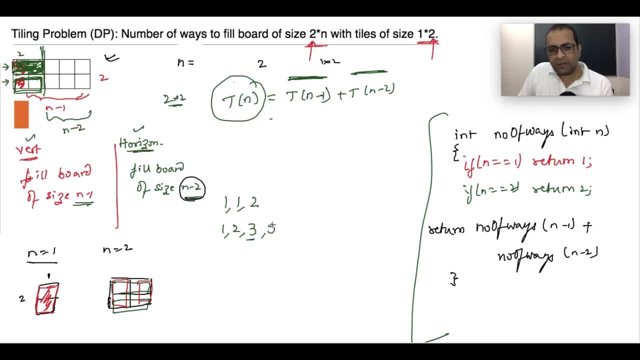 If length of the board is 4, then number of ways of putting the bricks is 5.. If length of the board is 5, then number of ways of putting the board is 5. And number of ways of filling the board is 8.. 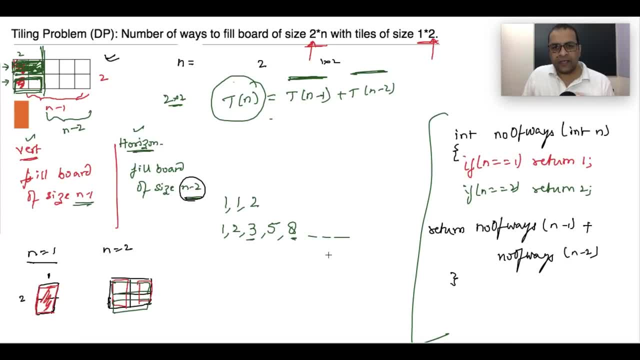 And so on. So this is all exactly equal to Fibonacci series. We have already seen the recursive, memoized and dynamic programming version of Fibonacci series, So you can see the code of Fibonacci series there. That code will be applicable here also. 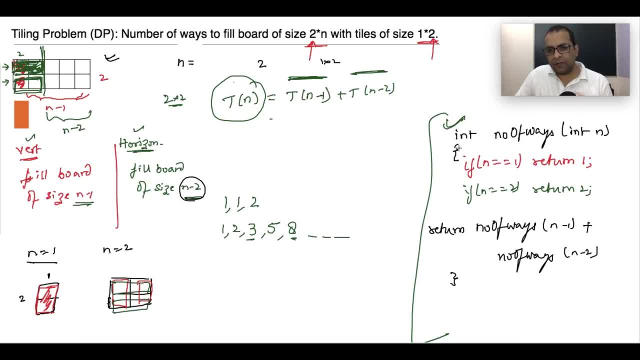 How much time is it taking? This way, if we are using the recursive solution, the time taken will be on the order of 2 days. So this way, if we are using the recursive solution, the time taken will be on the order of 2 days. 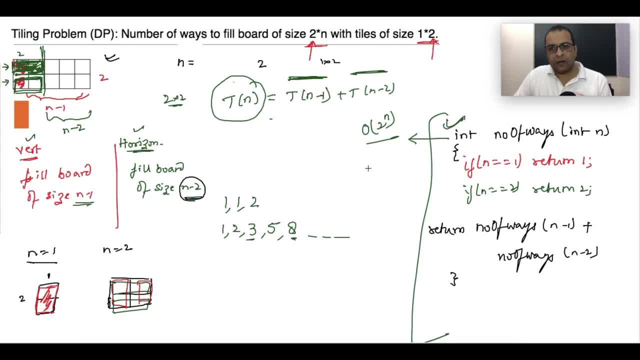 So this way, if we are using the recursive solution, the time taken will be on the order of 2 days Because there are overlapping subproblems. The dynamic solution for this problem is exactly same as dynamic solution of the Fibonacci series, where we keep two variables. 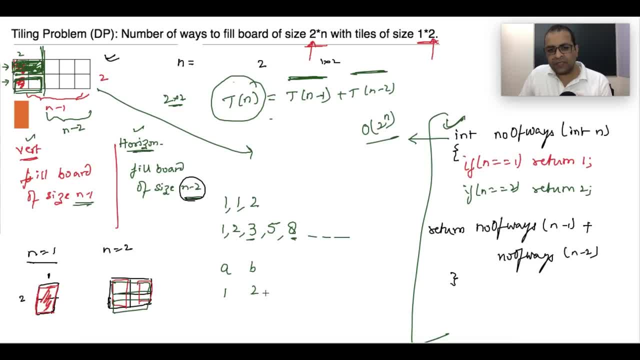 a, b. a is initially 1,, b is initially 2.. Then we take a third variable, which is equal to sum of a and b, which is 3.. Now a will be equal to b, b will be equal to c. 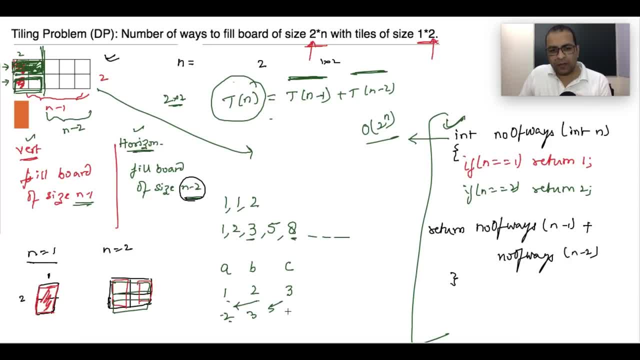 And we kind of recompute c again, So c is equal to a, plus b again, So c is equal to 5, and so on. All right, So that way the complexity of this problem can be reduced to. on the order of n.